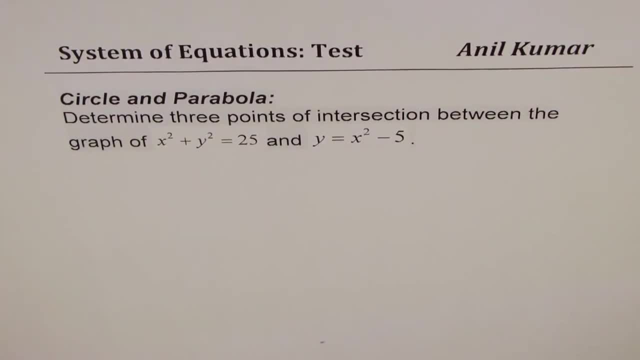 I'm Anil Kumar sharing with you a test question on system of equations. So we'll consider a circle and a parabola and we'll find their points of intersection. The equation is: determine three points of intersection between the graph of x square plus y square equals to 25 and y equals to. 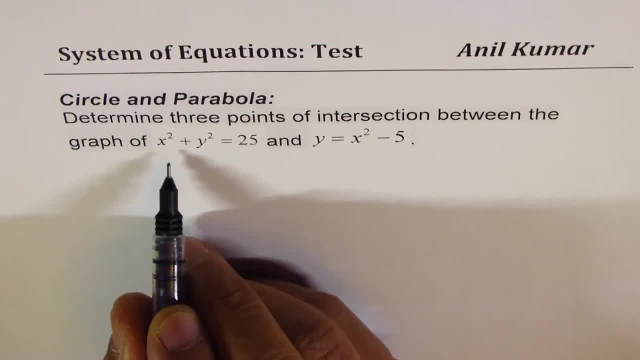 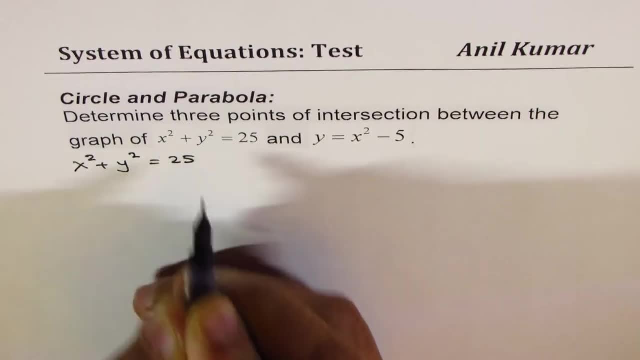 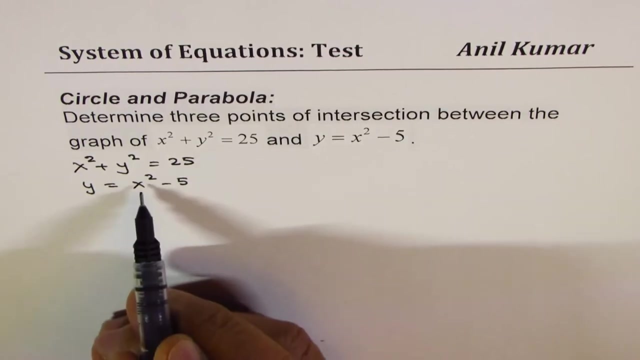 x square minus 5.. So we are given two equations here. The first one is of the circle, which is x square plus y square equals to 25.. The second one is y equals to x square minus 5.. Now we can isolate x square from the second equation. It gives us x square equals to y plus. 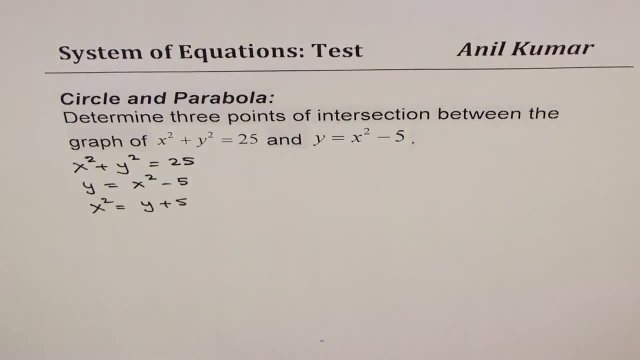 5, bringing this 5 to the left side. and now we can substitute from equation 2 the value of x square in 1 right. So now we'll substitute 2 in 1.. So that is to say we could write this as: y plus 5 plus y square equals to 25.. Rearrange. 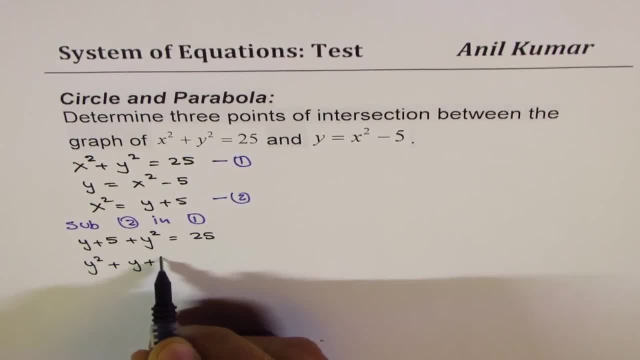 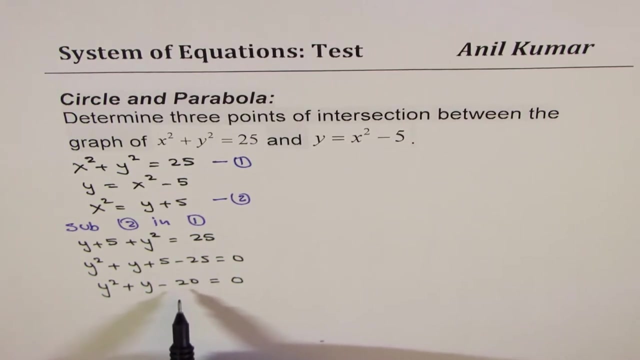 So we get y square plus y plus 5 minus 25 equals to 0, which could be written as: y square plus y minus 20 equals to 0. Now you could factor this: We are looking for two numbers whose product is minus 20.. Let's say two numbers, p and q, whose product should be minus 20, and the sum should: 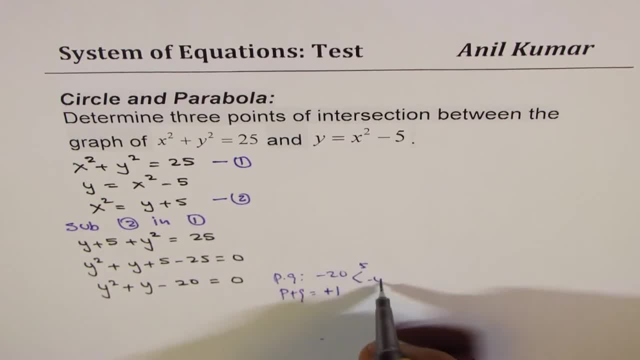 be plus 1. So the numbers are 5 and minus 4.. So this can be factored as y plus 5 times y minus 4 equals to 0.. Now that gives us two points. So let's figure out what these two points. 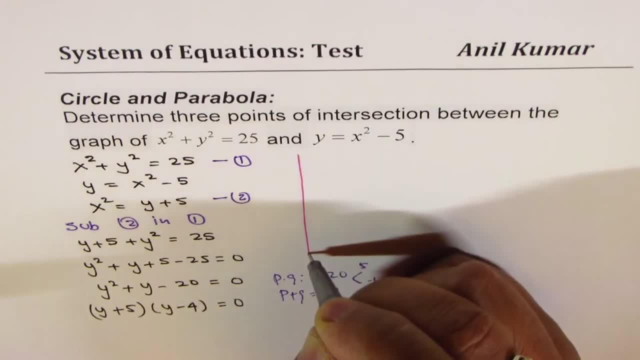 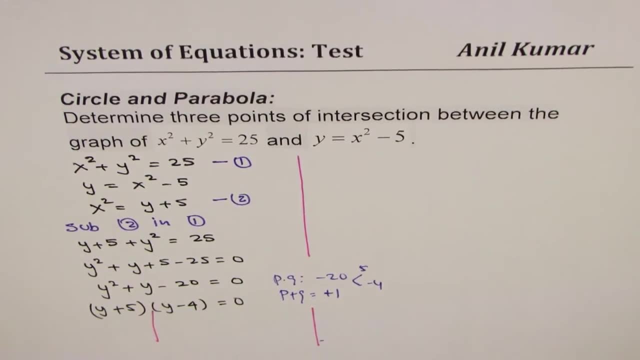 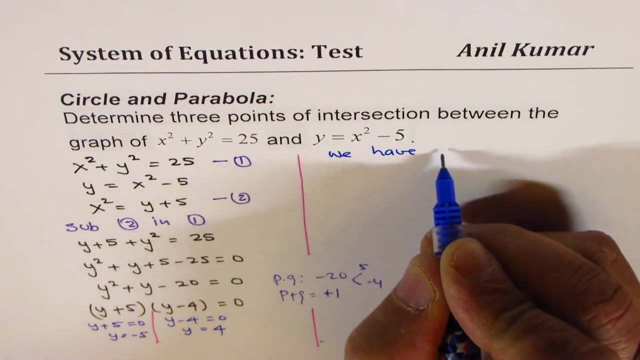 are by equating Each factor to 0.. So these are the two factors. So if I write y plus 5 equals to 0,, I get y equals to minus 5.. If I get y minus 4 equals to 0,, we get y equals to 4.. So we have two values: y equals. 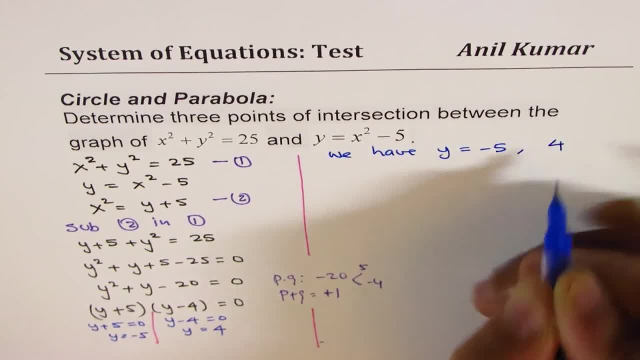 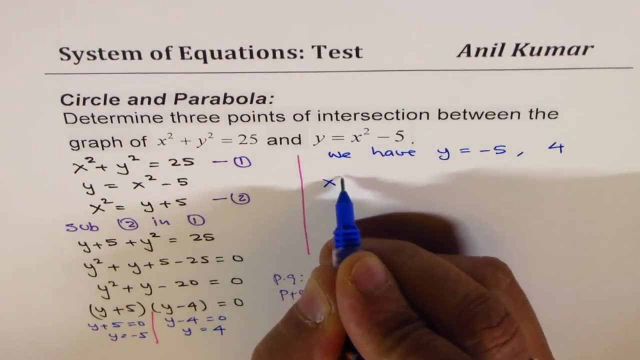 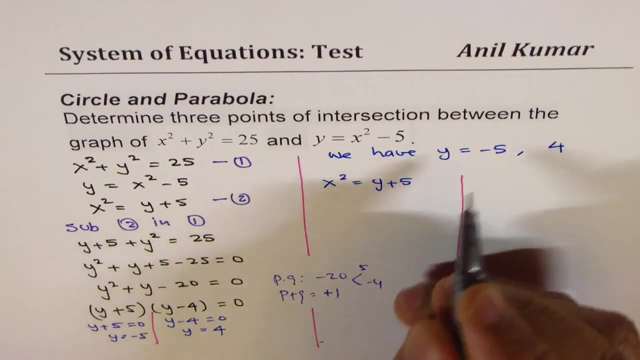 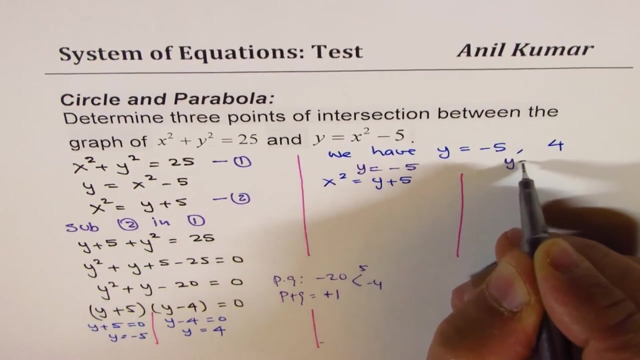 to minus 5 and 4, correct Each value. we should find the value of x. So we have this equation: x square equals to y plus 5.. So we will actually find both the x values, for y equals to minus 5 and for y equals to 4, right. 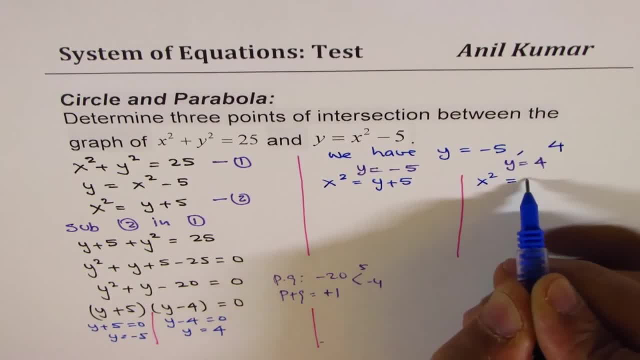 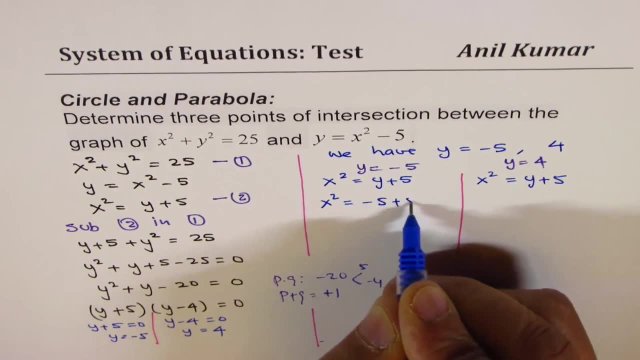 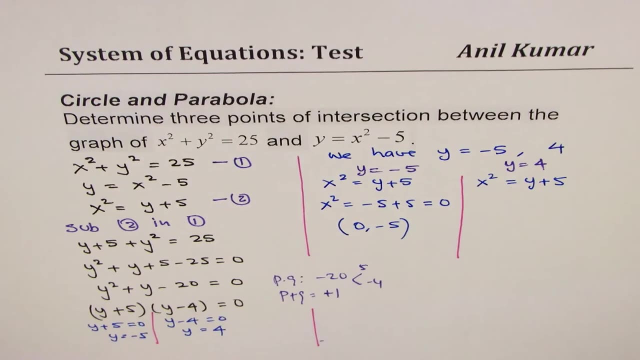 So the equation is: x square equals to y plus 5.. If I substitute minus 5 here, I get x square equals to minus 5 plus 5,, which is 0. And therefore the point is 0 minus 5.. So we get one point of intersection. If I substitute 4, I get x square equals to 4 plus 5, which is 9.. So x square is 9.. X should be square root of 9.. Whenever you do square root, you have to do plus and minus, And that gives us two points: plus and minus 3.. And therefore the coordinates of the x square equals to minus 5 plus 5, which is 0.. And therefore the point is 0 minus 5.. So we get one point of intersection. If I substitute 4, I get x square equals to 4 plus 5,, which is 9.. So x square is 9.. X should be square root of 9.. Whenever you do square root, you have to do plus and minus, And that gives us two points: plus and minus 3.. And therefore the coordinates of the x square equals to minus 5 plus 5.. And therefore the coordinates of the x square equals to minus 5 plus 5.. And therefore, 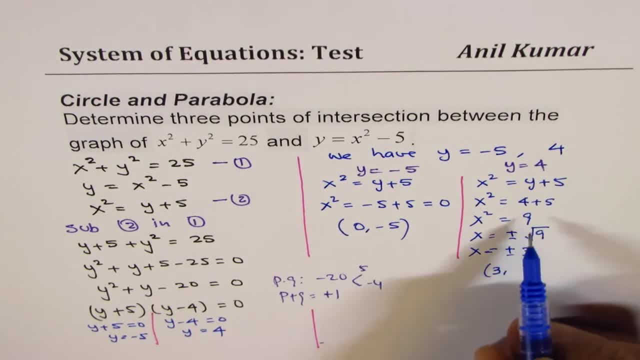 these points are 3 and the Y value is 4, or it could be minus 3 and 4. you get an idea right. so we have our solution and the answer here is: the points are 0 minus 5 and these two right, which is 3, 4 and minus 3, 4, correct. so that is how we. 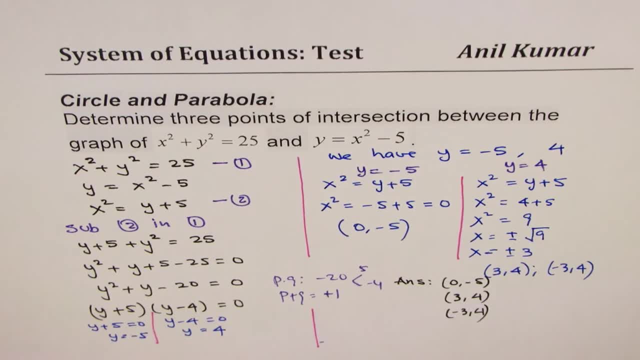 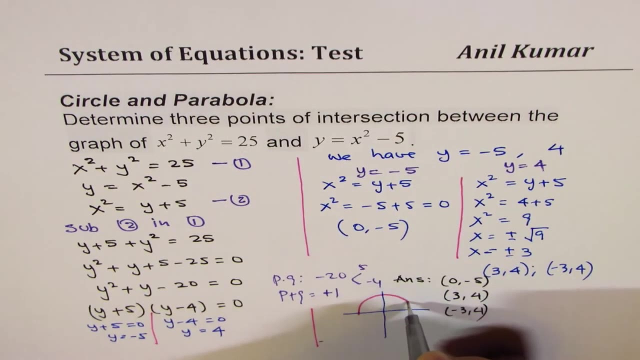 can get the solution to give you a picture as to how it should look like. so, if you actually sketch it, we have a parabola and a circle, so the circle here is x square plus y square, with the center at 0, something like this: my. 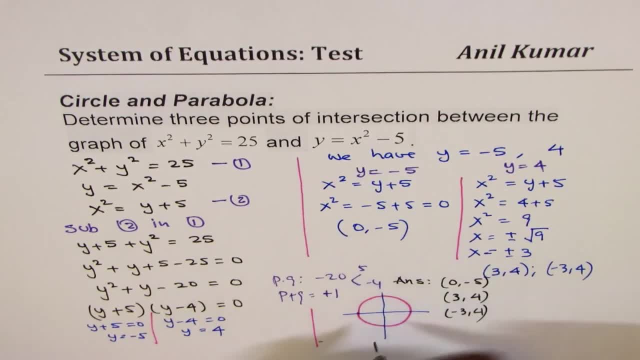 as far as the parable is concerned, X square minus 5. so this point is minus 5 for us. so we see that it intersect something at there, right? so it just is kind of a parabola which is like this: and these are the points of intersection.